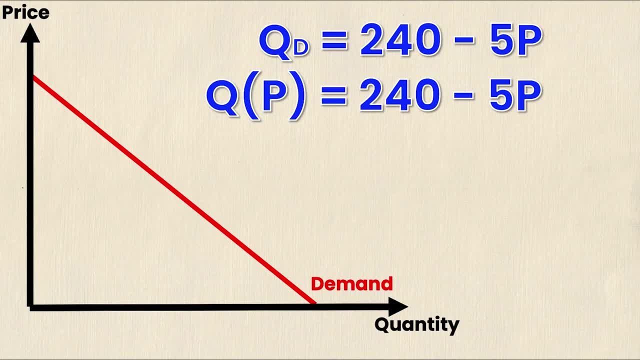 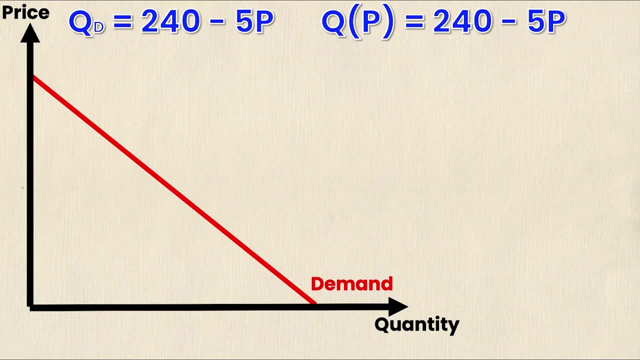 Q is the dependent and p is the independent variable, or that Q depends on p. That's the same thing. So if I wanted to calculate the inverse demand function, well, looking at this right now, I could tell you that the inverse demand function is: p is equal to 48 minus 0.2q. But the aim of this, 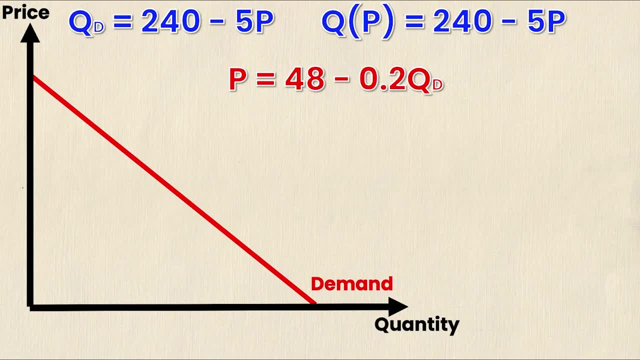 video isn't to simply tell you what the inverse function is, but rather how you can take the original demand function and turn it into the inverse demand function. And so we're going to do that step by step, starting by rewriting the original demand function. Q is equal to 240 minus. 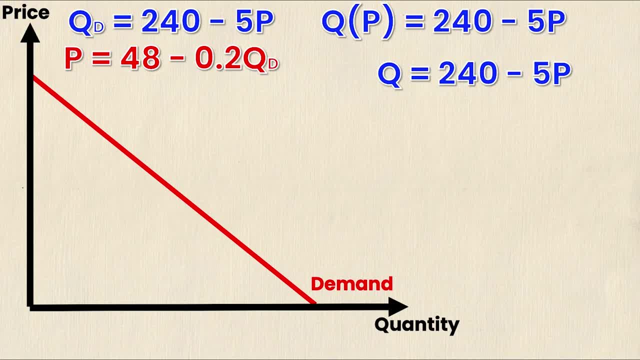 4p. So what I'm going to do is isolate for p instead of isolating for q. So now I want p to be the dependent variable and q to be the independent variable, And so to do that, the first step I'm going to do is switch the side of the equal sign that they're on. So the 5p is going to go to the. 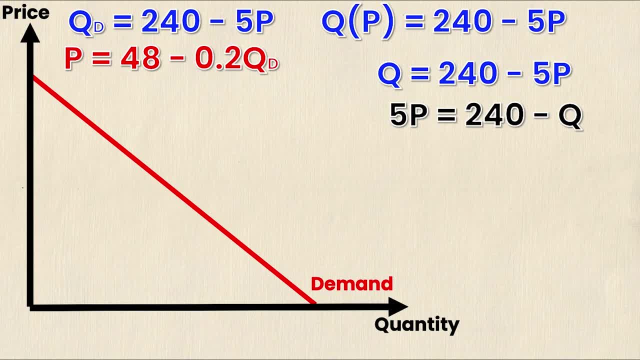 left side of the equal sign and the q is going to go to the right side of the equal sign. Now anybody studying economics should know the mathematics behind. switching sides of the equal sign ends up switching the sign of the coefficient. So now my 5p is equal to 4p. So now I'm going to do the. 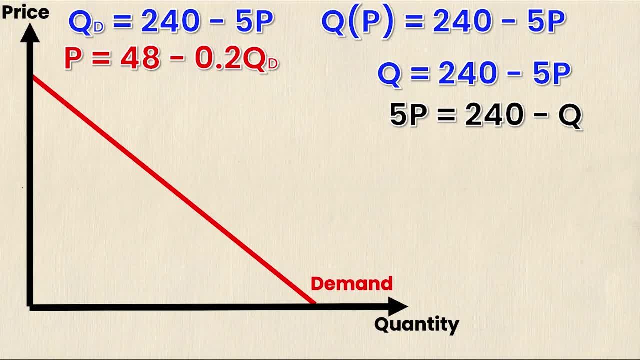 same thing for the 4p. So 5p is positive and my q is negative. Now you'll see that p is not quite by itself. It's being multiplied by 5.. And to get rid of that multiplied by 5, I'm going to divide. 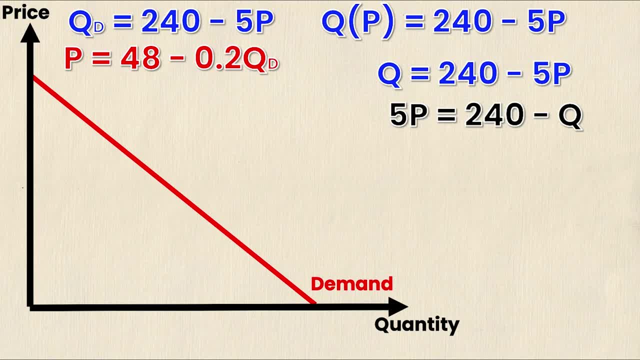 every term by 5.. So 5p divided by 5,, 240 divided by 5, and q divided by 5.. That yields me this next line: p equals 240 divided by 5 minus q over 5.. And you might be saying, well, where's the 5? that? 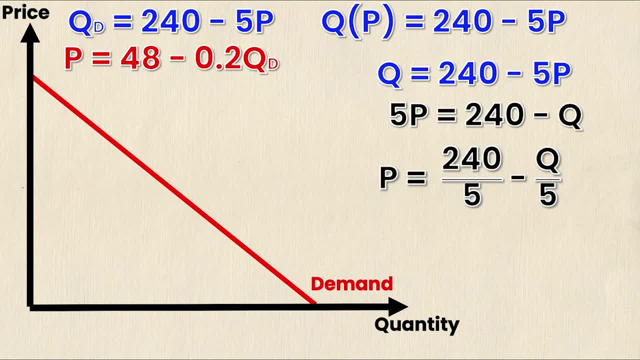 was on the left side of the equal sign. Well, 5p divided by 5 is just better. So I'm going to simplify this further by solving for 240 divided by 5, which is 48. So now I have: p is equal to 48. 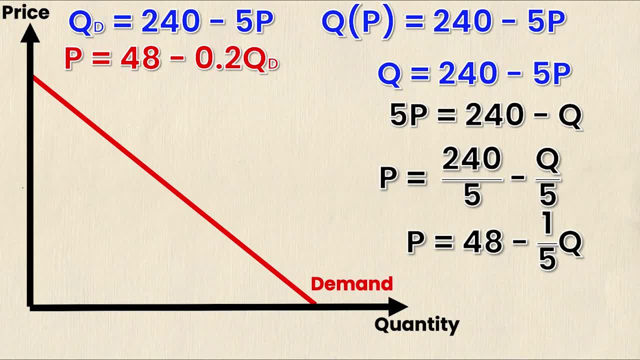 minus one fifth q, And you might say: well, the previous line was q over 5.. Well, q over 5 and one fifth q is the exact same thing. Now, you could just leave it as this, but a lot of people don't.